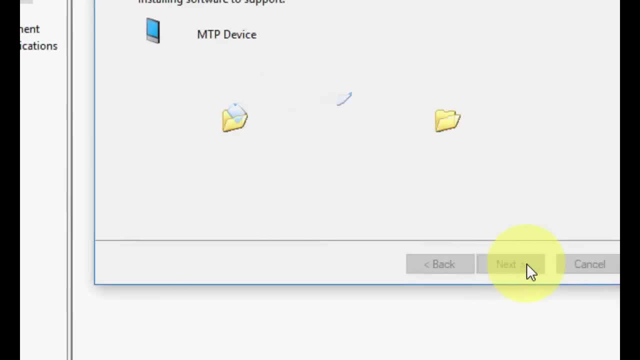 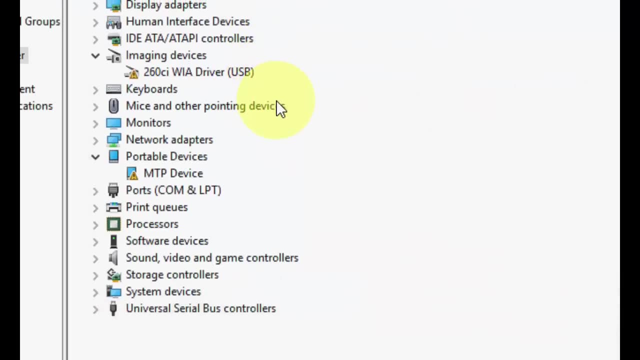 MTP devices and click next. next and it will install your supporting software. So this is the easy way to install your missing devices from device manager. So here you can see how to install your devices. update. you're gonna need to do. 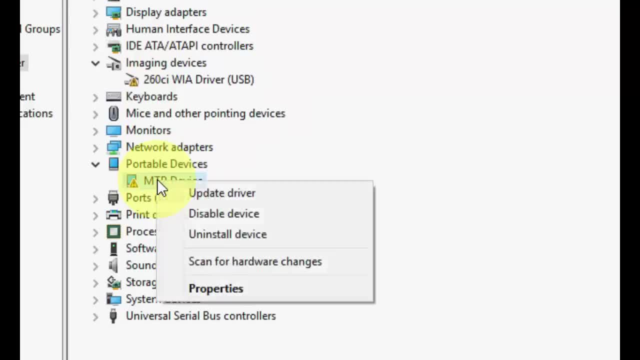 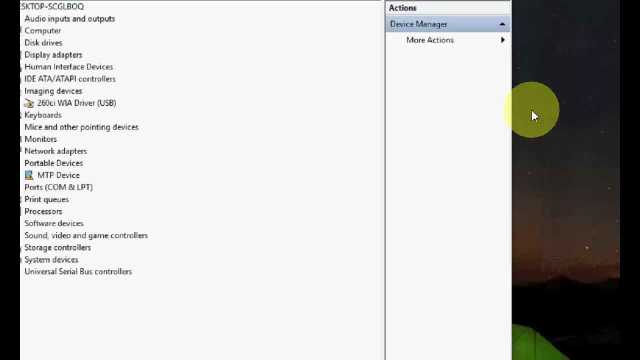 device manager and after this you will get. you need to update this driver to our suitable software to your hardware. that is, guys. I hope this will help you. time for watching. catch the next video. please like, share and subscribe. thank you very much. 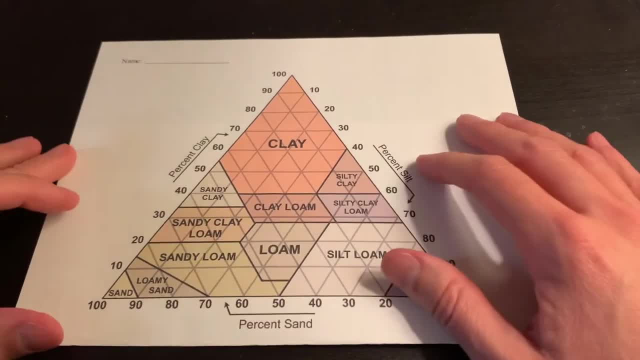 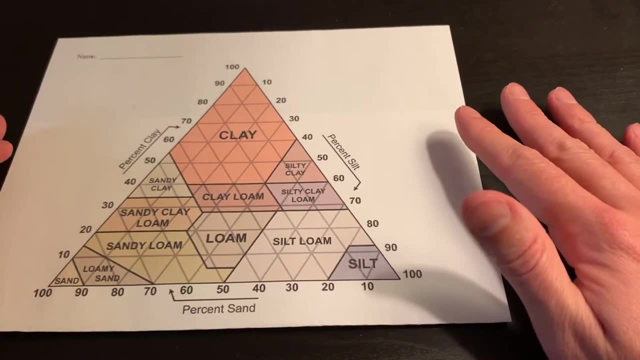 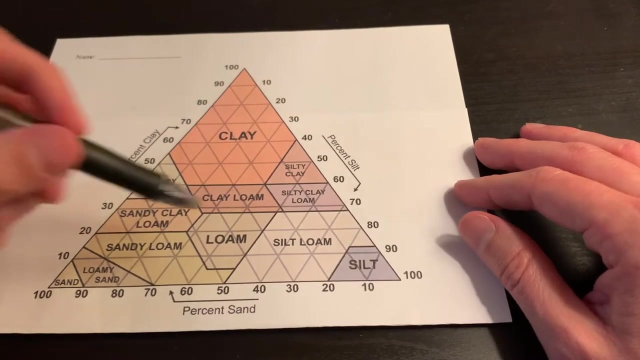 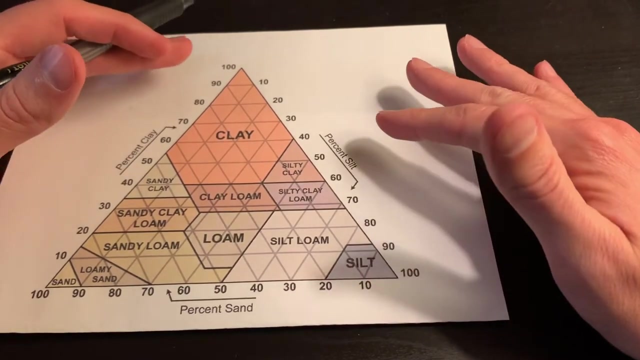 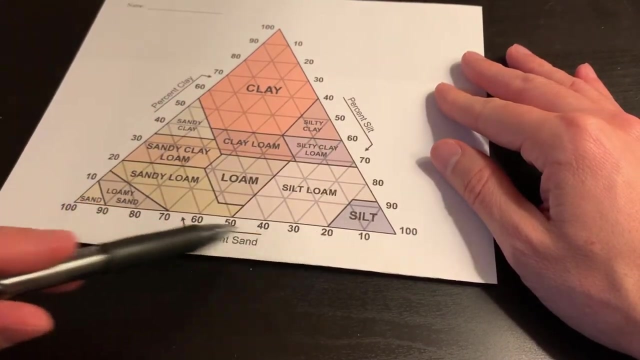 Let's take a look at this soil texture triangle and we'll talk all about how to use it to place you somewhere between sand, silt and clay. Now remember, this is a spectrum and if you had a spectrum between two points, you're going to be somewhere on a line. But because this is a 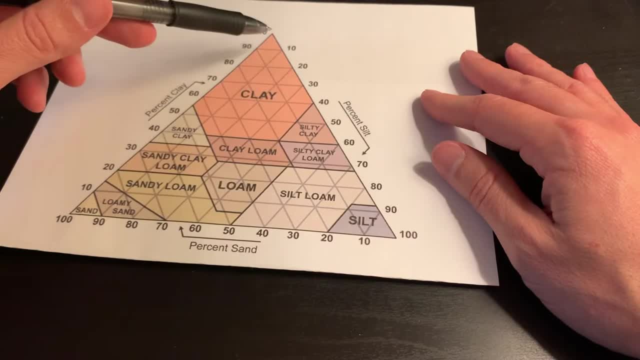 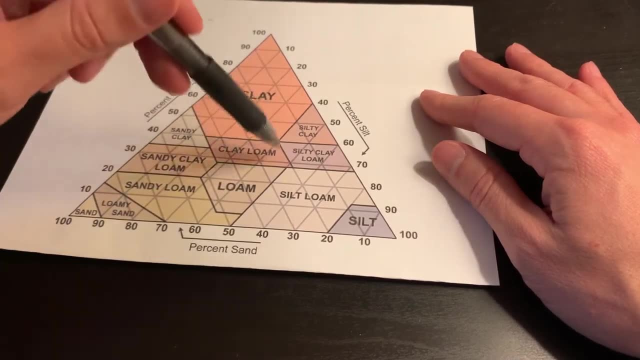 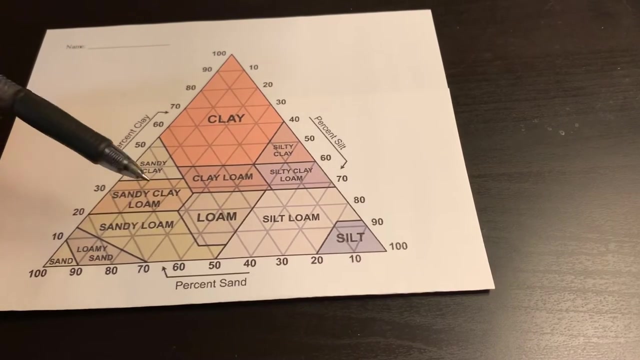 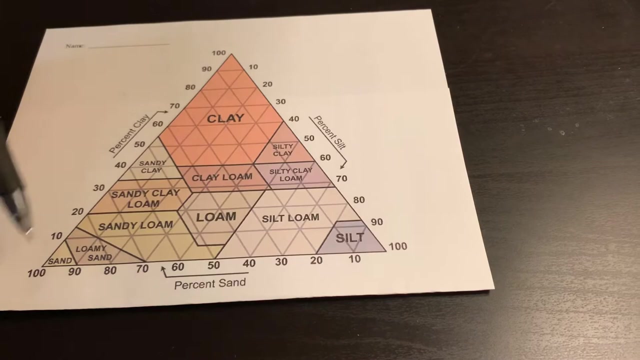 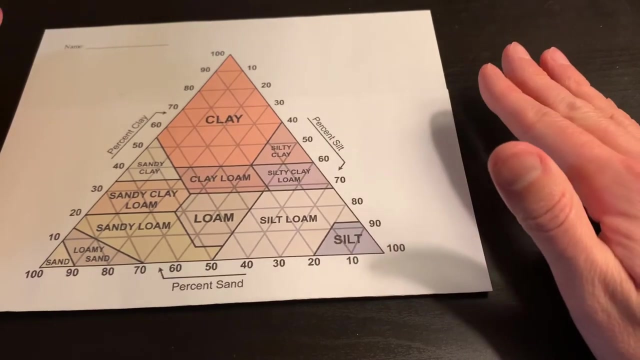 spectrum between three extremes. it makes a triangle, So we're going to be somewhere along this triangle with each and every soil type. It can be a little bit tricky to read this because we've got numbers. So we have 0 to 100,, 0 to 100, and 0 to 100 on all three sides. And so when you find out what 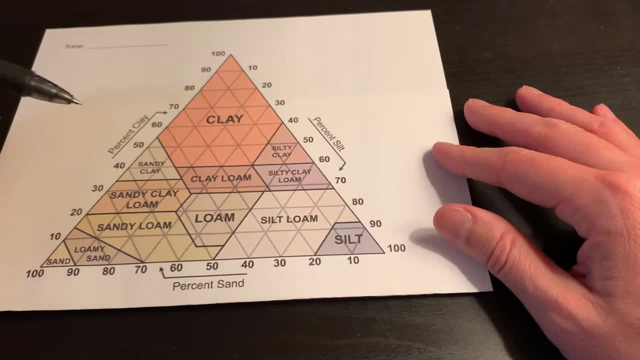 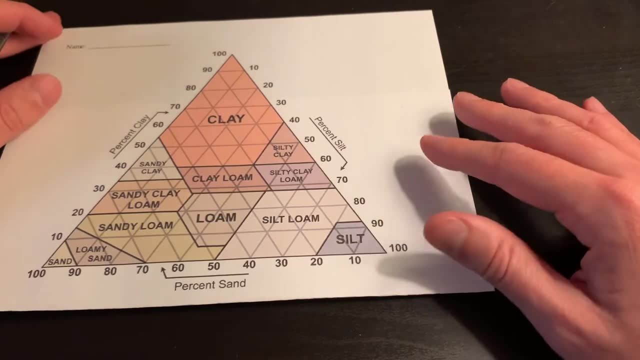 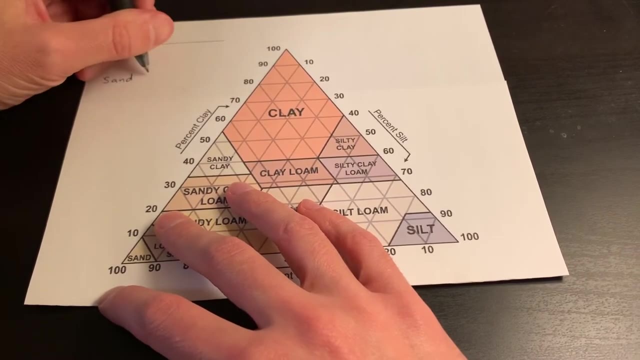 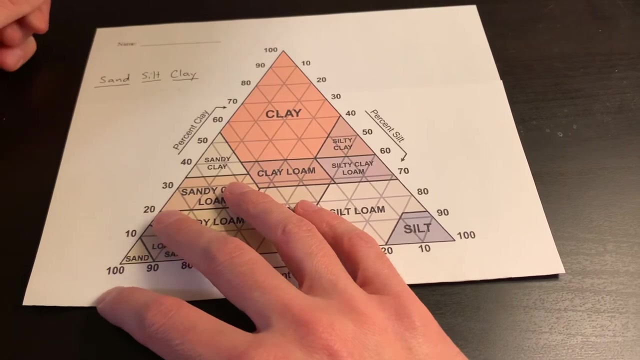 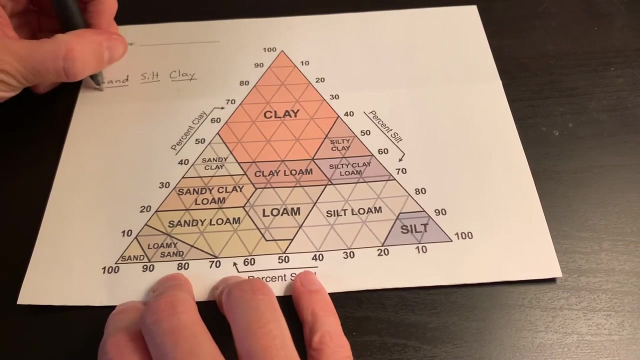 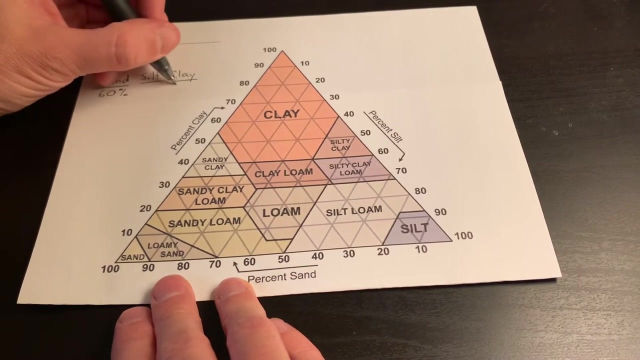 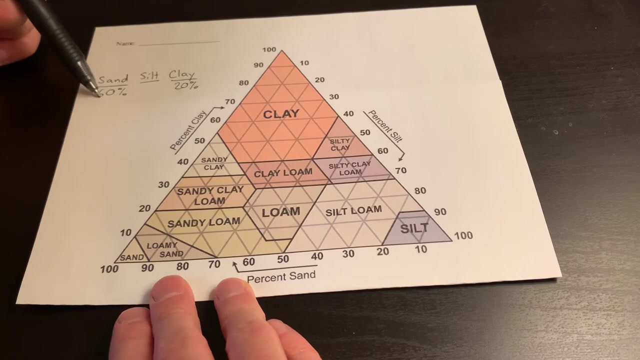 percentage of each of these soil separates you have. you need to make sure you're reading it the right way. So let's just say we find out that we have sand, silt and clay If we make a mistake at the primary нрав or numeric.